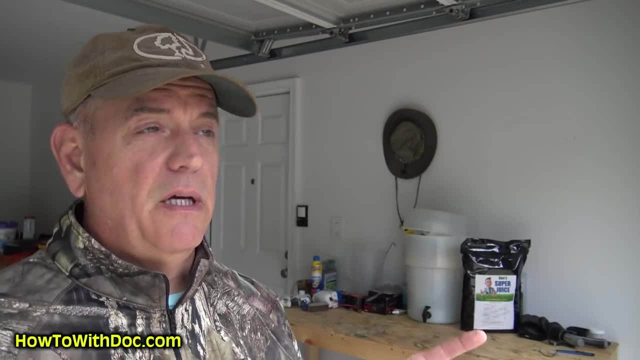 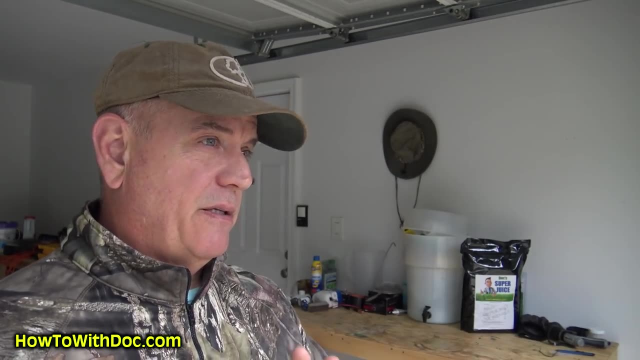 short on my phosphorus, I put down some 10,, 10, 10.. Uh, last week I put it down a little bit of 10,, 10, 10.. Now my lawn is only getting SuperJuice, by the way, that's it. And uh, I put a little 10,. 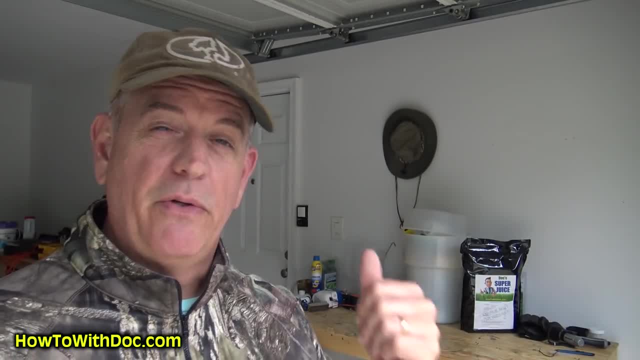 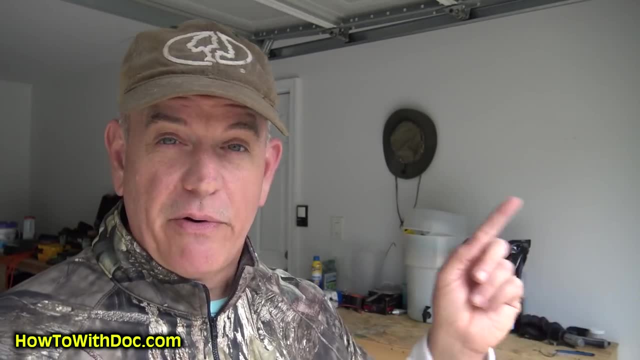 10, 10 to correct my phosphorus, And I told you I was going to put down a spray. So I'm going to do the phosphorus adjustment, a little extra iron and the SuperJuice all in one. That's what I'm going to do today. Uh, I was going to show you a little irrigation hack that I did where I 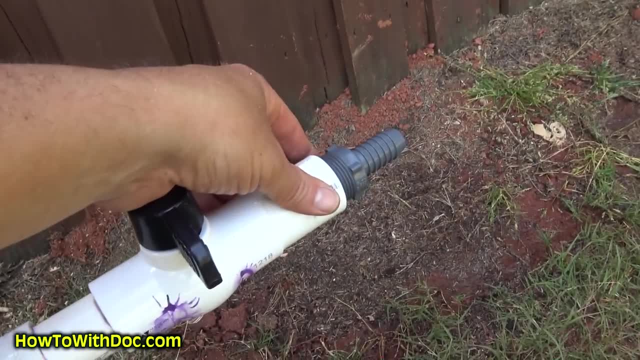 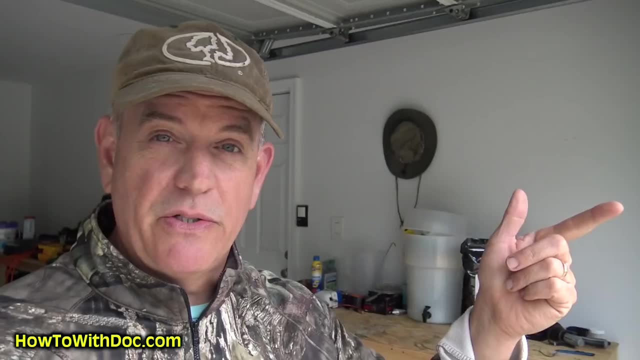 uh, have a garden hose spigot on the right side of my house. They're all over on the left side and I have a slab foundation so I can't access it. So I tied into my irrigation system and put a sprinkler head. but that's too complicated, So click that subscribe button, So you know. 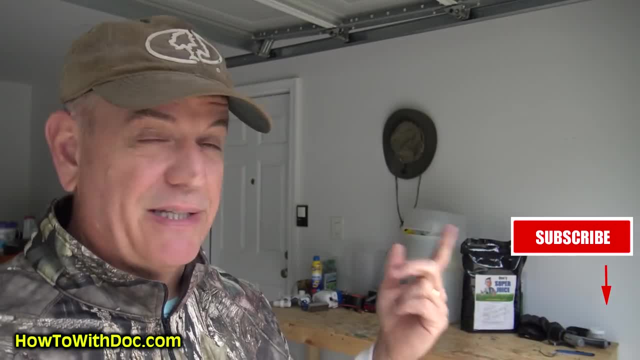 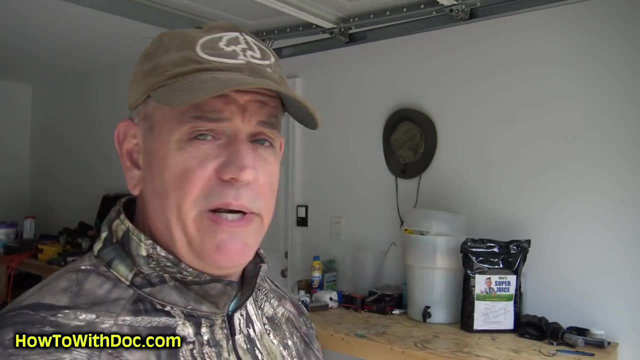 when I put that irrigation hack in. it's pretty cool if you want to see it, but it's kind of dangerous because of the high PSI. Man you talk about deadly, It's a deadly PSI, It's high. So, anyways, uh, I use liquid iron. 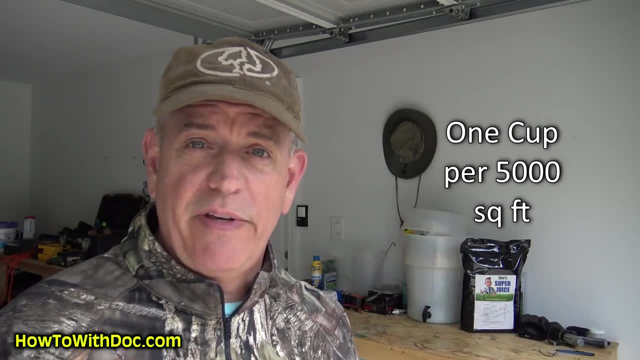 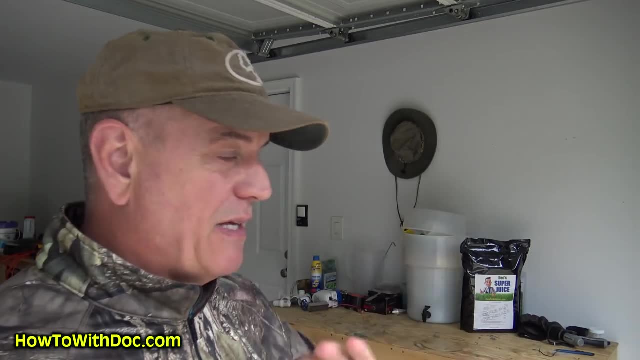 I put about one cup eight ounces for about 5,000 square feet. In case you're wondering, that's the amount that I use. I'm doing my own phosphorus readjustment. Uh, that's really doesn't matter to anyone, but let me tell you what. if you want a really really dark, green lawn, 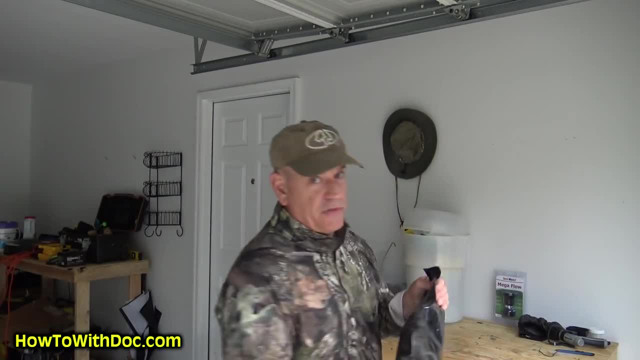 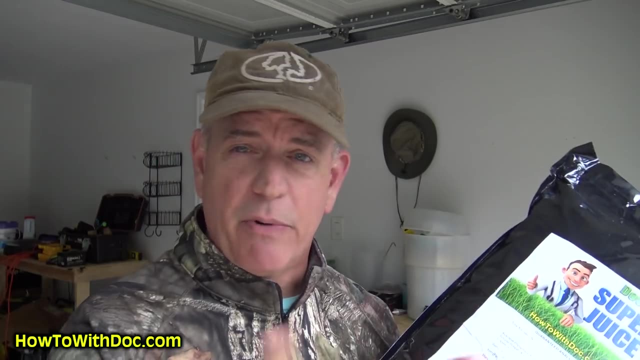 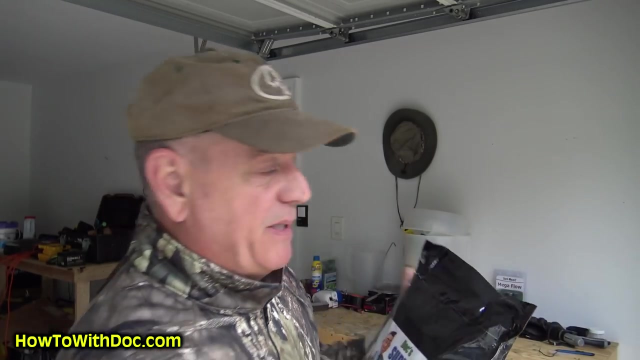 you can add iron Now SuperJuice. Now, SuperJuice is a complete and balanced formula. It already has a two or two and a half percent iron already inside of it. It's a powder. You mix it, spray it on your lawn and it's a powder. So you're putting out a very, very small amount of nutrients. It's. 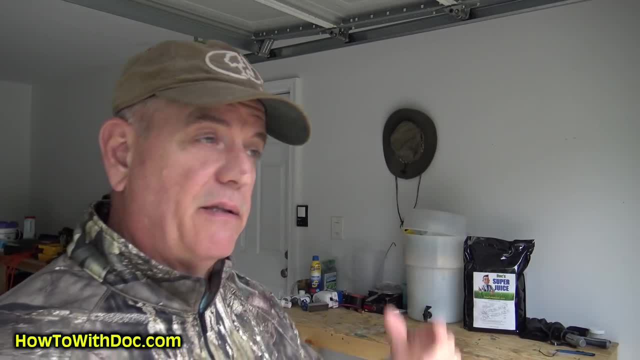 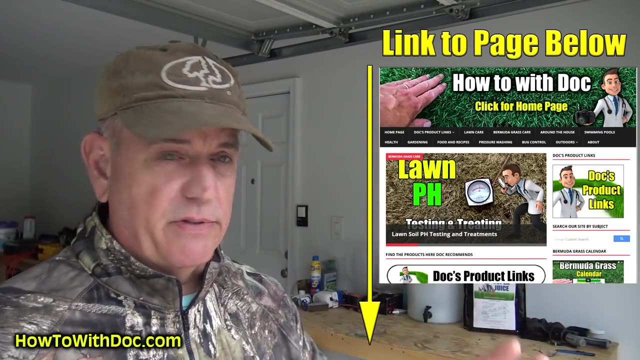 really designed as a supplement, So so if you really want to bump it up and add some additional iron, you can add liquid iron to this Um. in the description down below I'm going to have a link to a page and on that page I'm going to have several things. I'm going to have links to the 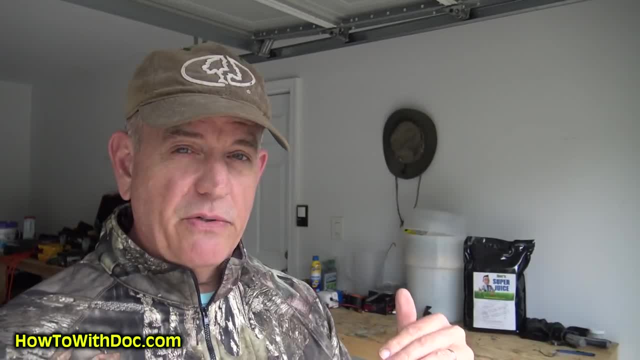 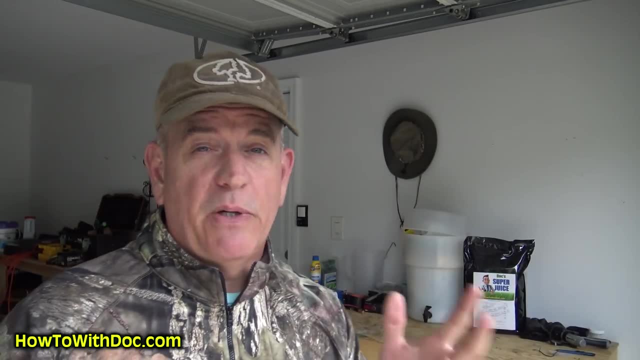 products that I'm using: the SuperJuice, the iron and everything else Plus. I'm going to have additional resources If you want to read them from universities and turf magazines and that kind of stuff about the benefits of iron. So the cool thing about iron is you can use iron to green up your lawn instead of nitrogen during stress periods. 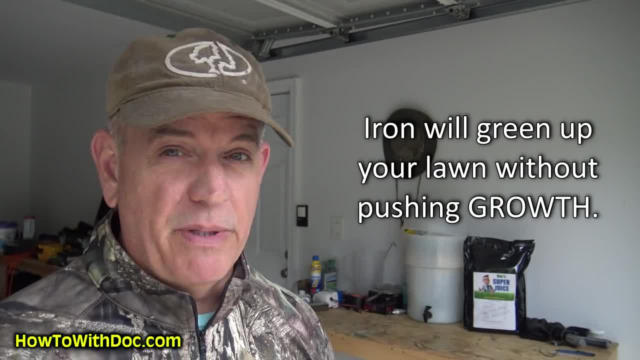 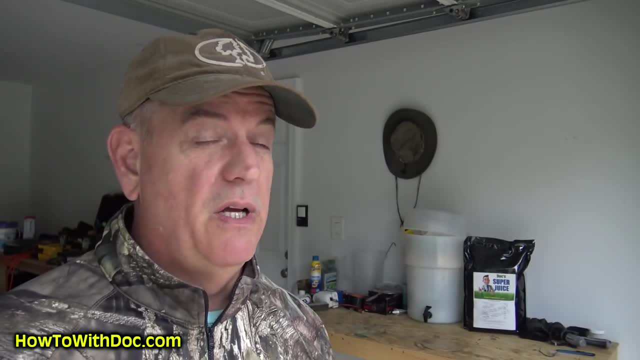 So you could put a whole ton of nitrogen on your lawn, but then your lawn is going to grow like crazy, It's going to use all this energy And if the heat comes in, if it stops raining, it's going to be under a lot of stress. So one little trick is to add some additional iron, and you're not. 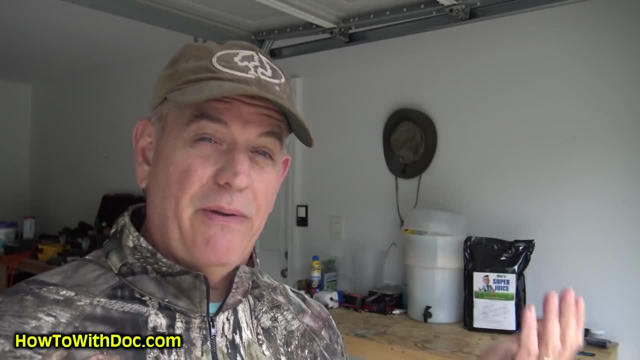 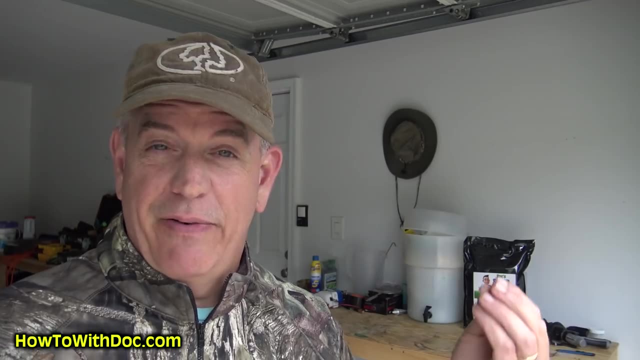 pushing the growth of your lawn during stress periods. So that's a cool little trick. Now you don't want to put a huge amount of iron down, because you can actually turn your grass kind of gray or even black sometimes, But again, using this method, putting down about one. cup or eight ounces per 5,000 square feet is plenty as a little supplement to boost up the SuperJuice. I like to do it every once in a while. Now this will be my sixth treatment, so I haven't done anything extra. This is the first iron extra iron treatment I'm doing. 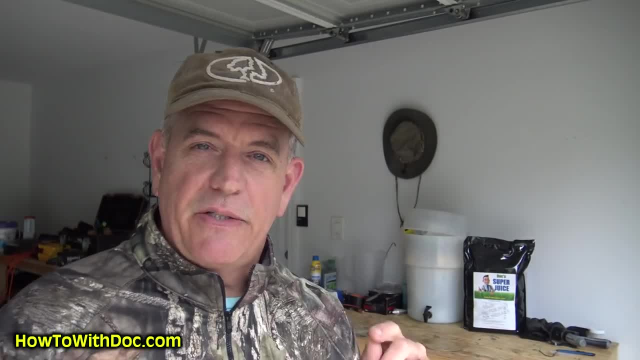 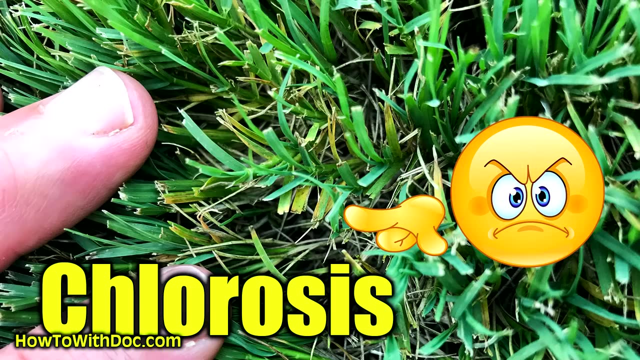 So, and I'll do it maybe once a month. The other thing is is if you start to have yellow, what's this? But if you start to have like yellow tips all over your yard, sometimes it's a nutrient deficiency, Sometimes it's a pH imbalance. but a little bit of iron can also help that too. So if 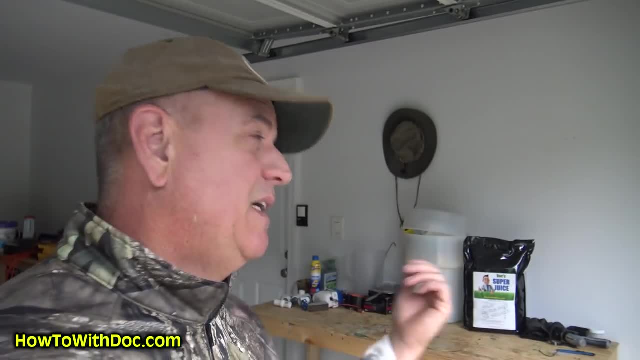 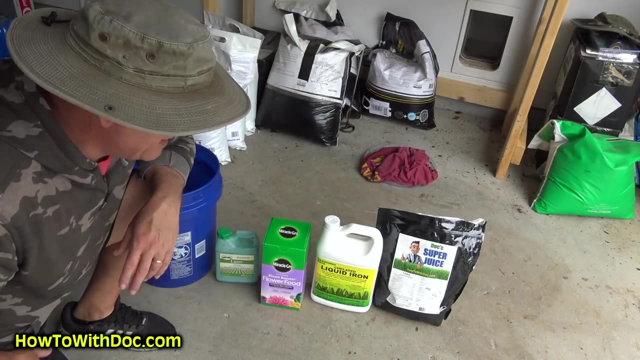 you start to see yellow blades of grass all over your yard. you can hit it with a little bit of iron until you figure out what's causing that problem. Okay, so what am I doing? This is not something the average person would do, but let me show you what I've got First. I've got, I've got. 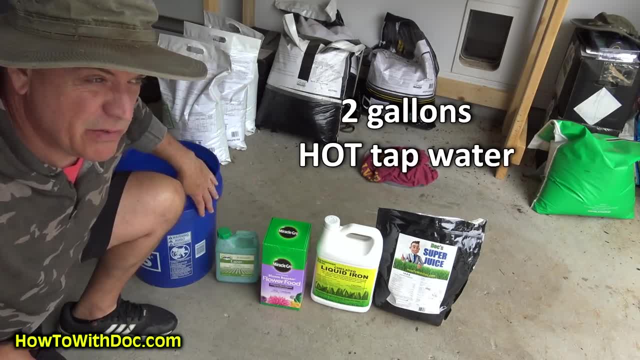 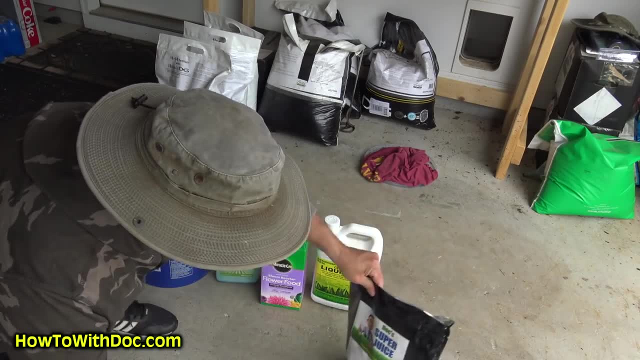 17,000 square feet, So I've got about two gallons of water. Again, the amount of water isn't important, It's what you put into it. that is important, As long as you apply everything that you put into the water to the lawn. that's what's. 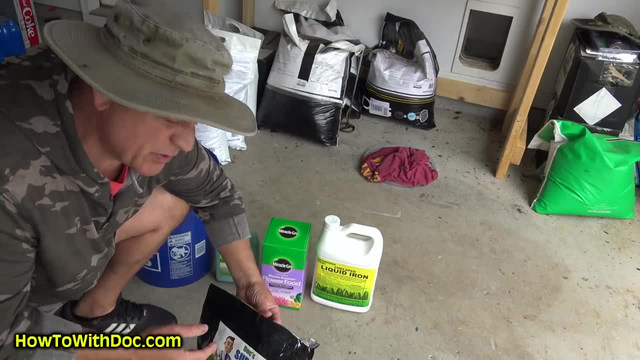 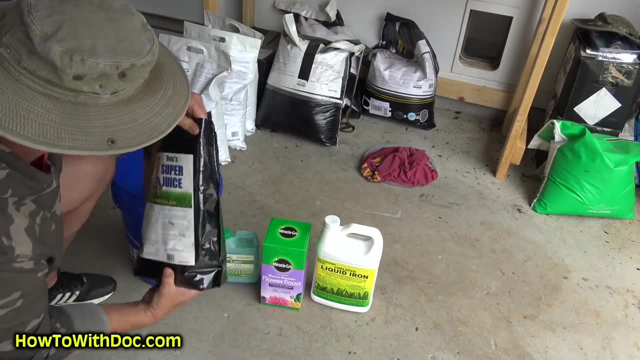 key. I've got about a fifth of a bag of SuperJuice, So this is about for me. a fifth of a bag puts out about a 7-1-2 ratio, So I'm going to put that in there. I like to put in every once in a while. 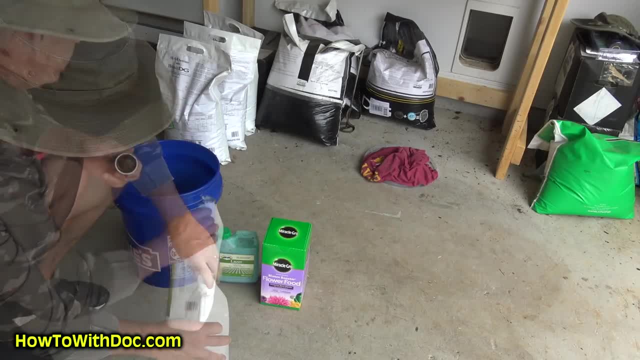 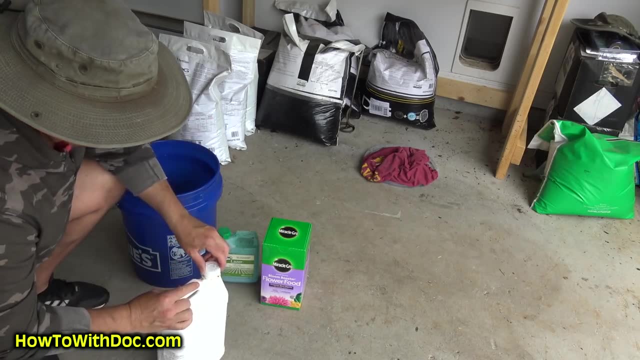 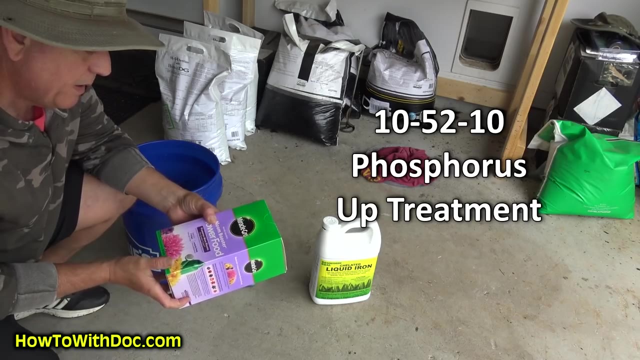 just a little boost iron. I'll put about a cup in there A little extra iron. give it a little blue color for the iron. This is the adjustment treatment. Now this is a 10-52-10.. So if this is four pounds, 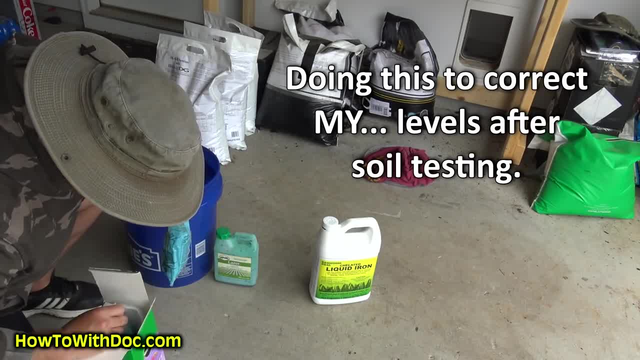 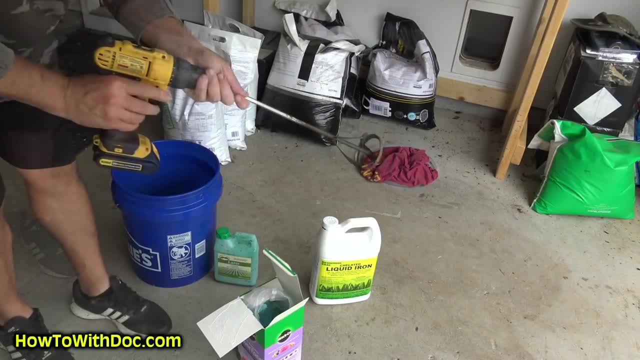 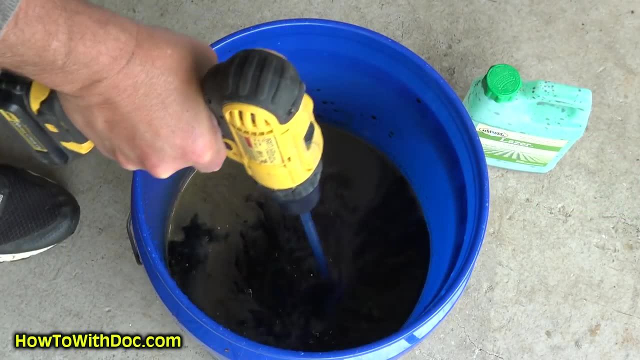 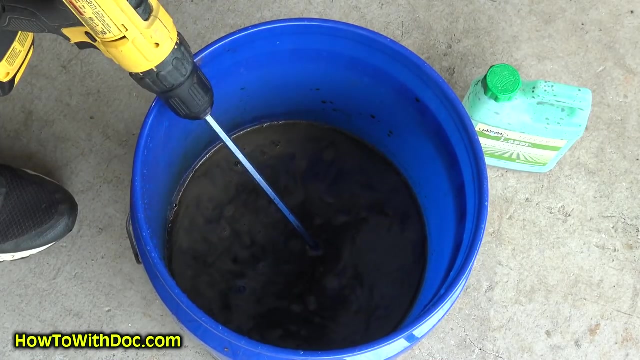 50% of this is two pounds. So there's one, two, three. there's three packs in here. I'll put one pack in. I like to leave it Again. this is hot water. I'll leave it for a few minutes. 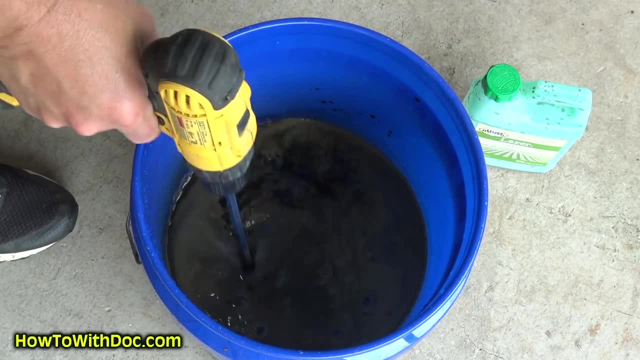 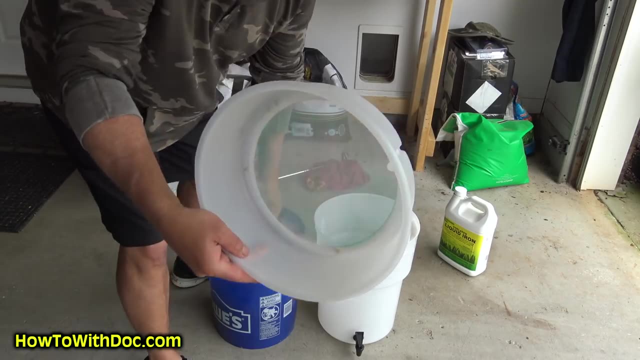 about five, 10 minutes, come back, stir it one more time and that'll be it All right. So I use a tea pitcher because I have to spray three lawns And I just take about a 400 mesh screen. 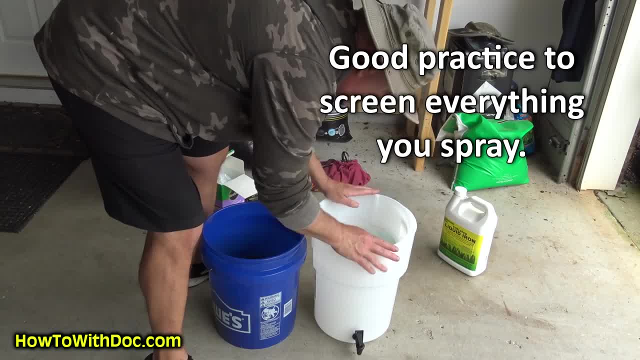 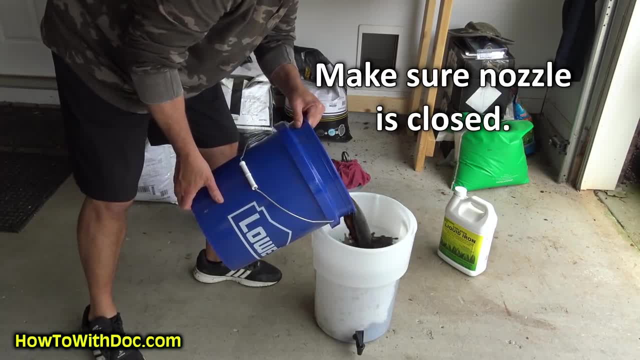 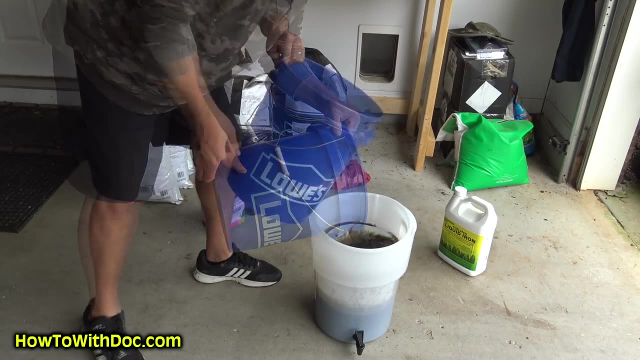 Okay, Not 400 mesh, 400 micron. I put it here And then I'll just go ahead and just pour it in. Now, if I have any humic left in here, what I'll do is I'll get the garden hose. 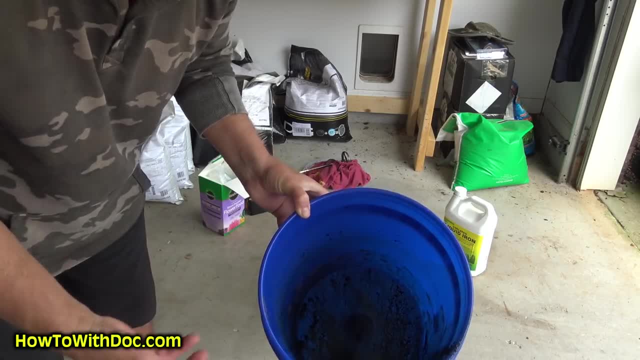 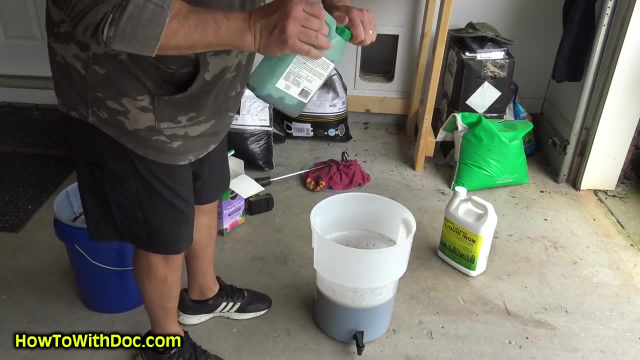 and I'll rinse this into my shrubs and gardens around. That's what I do with it. Now I'll take my dye, Which is the last thing I do, Almost out of green, So I'm going to use a little green. 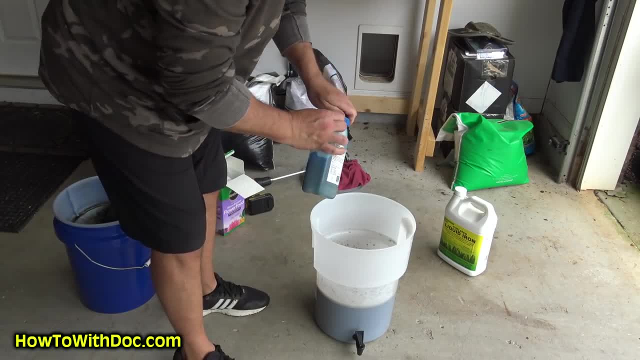 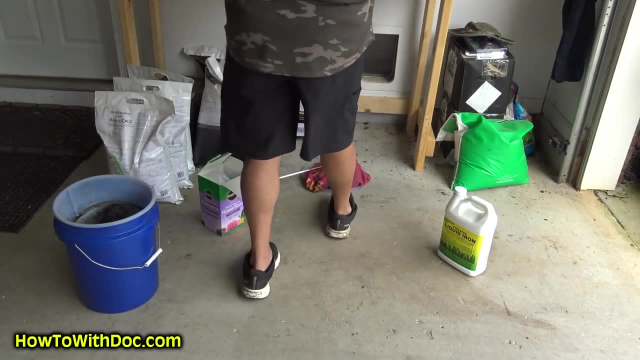 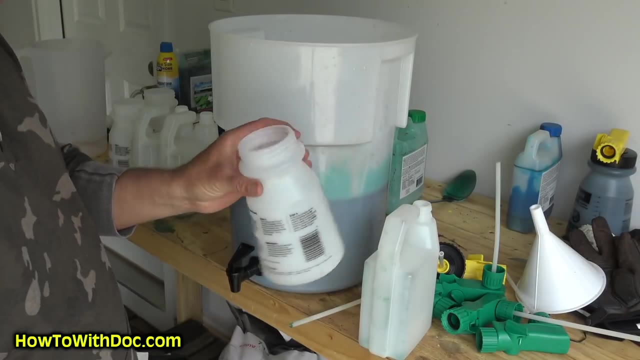 And I'm actually going to use a little bit of blue too, just for the heck of it, And I stir that up. So people ask me: do you prefer the yellow or the green bottles? The yellows are easier to clean out, but the yellow sprayers can be a little bit more touchy, I guess. 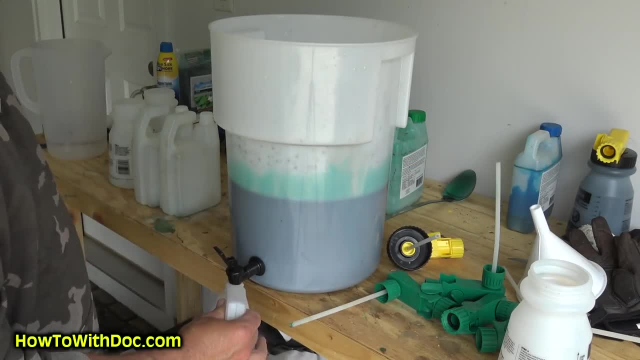 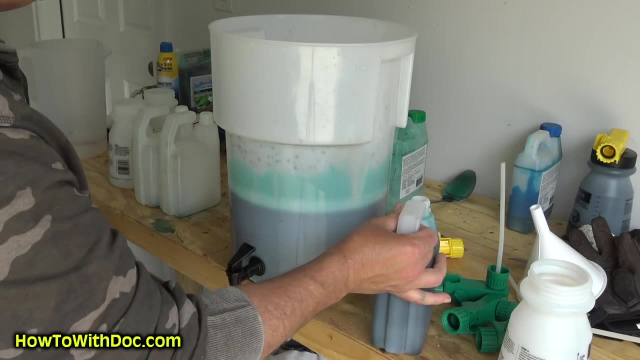 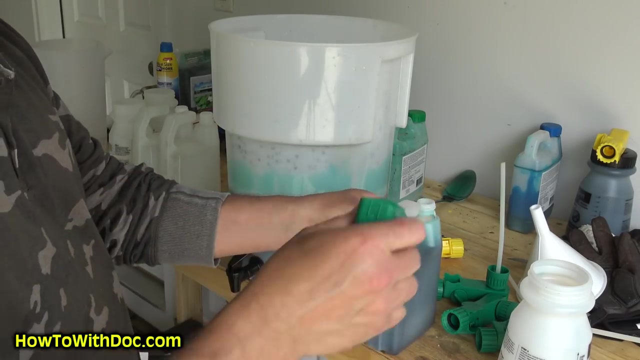 So I'll start off by using all green. Before you do this, make sure your bottle is in the off position, because you're going to be squeezing the bottle and that hole will be open There, just like that. She's ready to go. 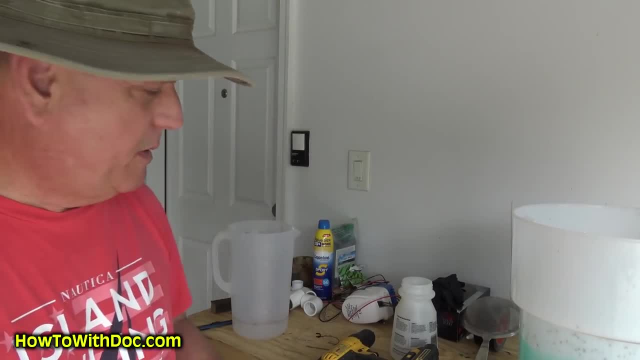 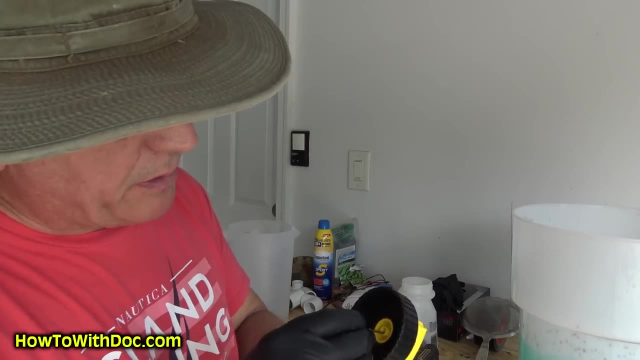 So if you watched one of my earlier videos, I talked about taking a 3- 32nd drill bit. If you're having sprayer troubles, take a 3- 32nd drill bit and go in here and just open up that hole, a little bit like with a pair of pliers or vice grips. 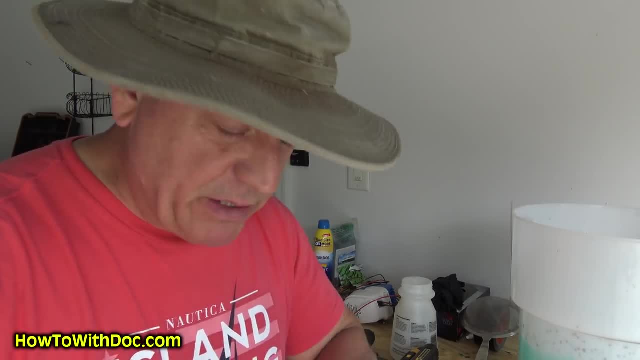 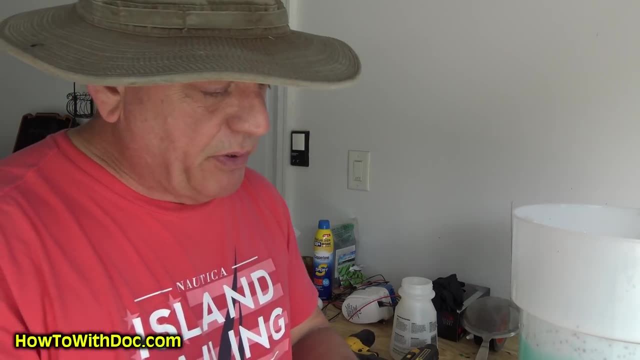 Or you can drill it slowly. You're not trying to ream this hole out because it'll spray too much. But here's another thing One of my viewers actually said something about. he put a breather hole in the top of his bottle and that got me thinking that there is another. 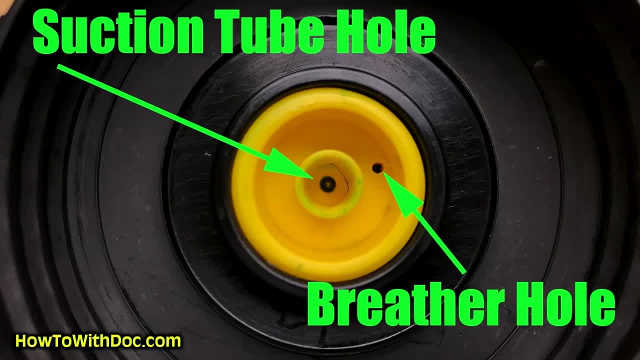 tiny on these yellow ones. there's another tiny little hole here. There's another tiny little hole here, And you don't want to leave a tiny little hole in there, And that's what I do. I'm just trying to make sure there's no holes there. 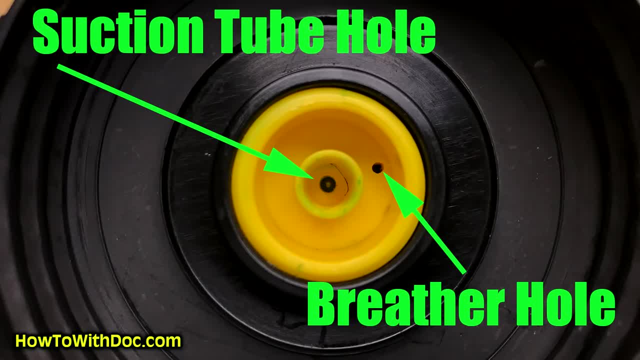 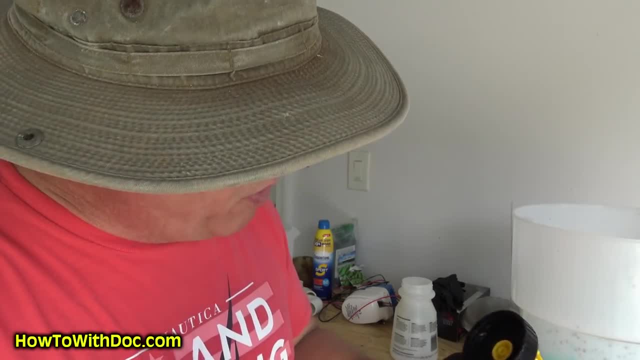 And you don't want to leave a tiny little hole in there, And you don't want to leave a tiny little hole in there. That's a breather hole. So I got an even smaller drill bit and what I'm doing is I'm opening that breather hole. 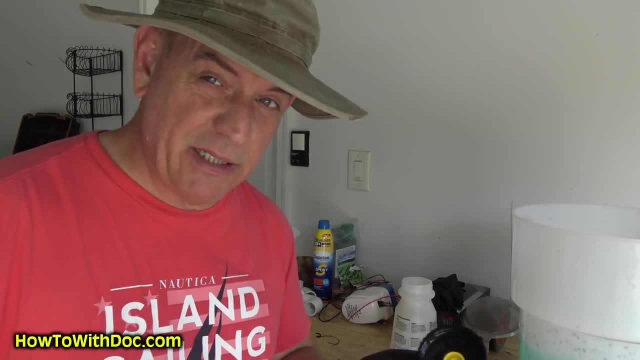 up just a little bit just to see if that helps. Now he said it made an amazing difference, but I think what he did is he drilled a hole in his cap, which you got to be careful because if it tips over it's going to spill. 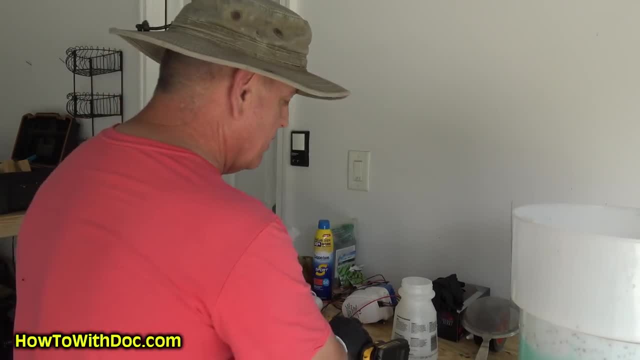 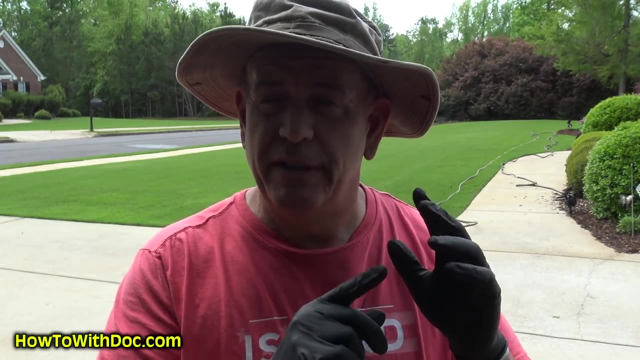 So I'll check this sprayer out first and we'll see how it works. Hey guys, so I did check out that sprayer with the extra little breather hole that opened up a little bit, and it works really well. So I don't know if that's a cure or not. 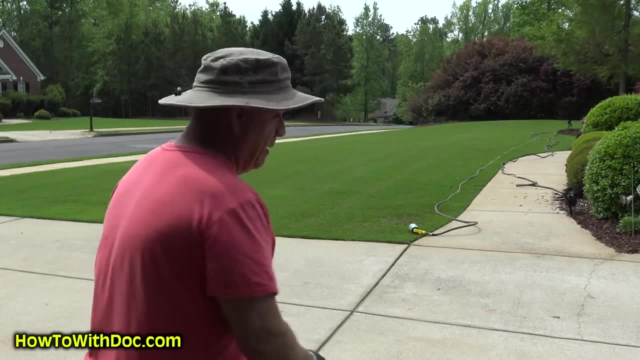 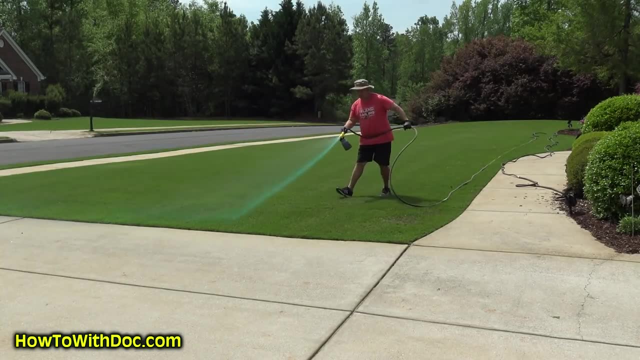 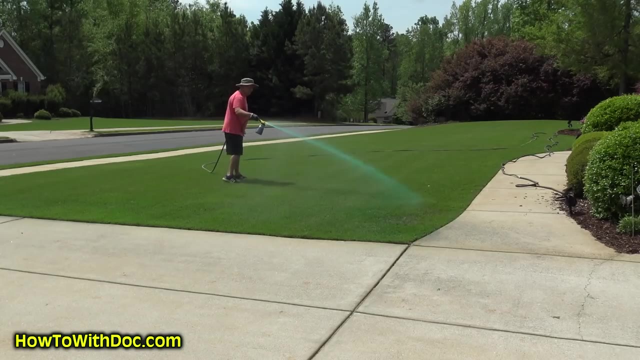 I don't make the bottles, So I'm going to go ahead and spray. I'm going to have to watch pretty quick, because this stuff's really coming out now. Hey guys, so I've been doing a lot of online shopping lately. And I've been. I've been feeling really low at the same time Feels all right, then I'm wrong, Hoping I'll be fine. But I get up. I always do. I never think, I always do. Never thought I wouldn't jump. oh, what a fool. 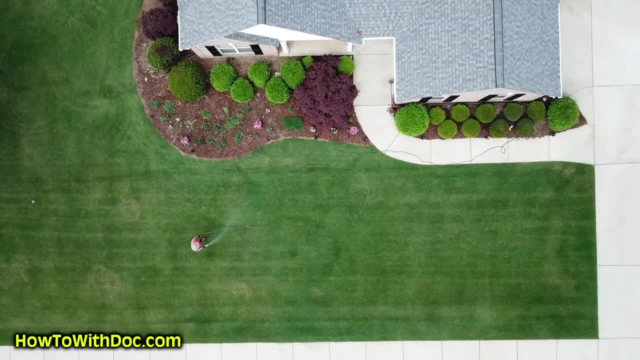 But if I fall, I would get up again, So I'm going to go ahead and spray that up. I'm going to go ahead and spray that up just to see if it works. Okay, so I've got that done. I've got it all done. 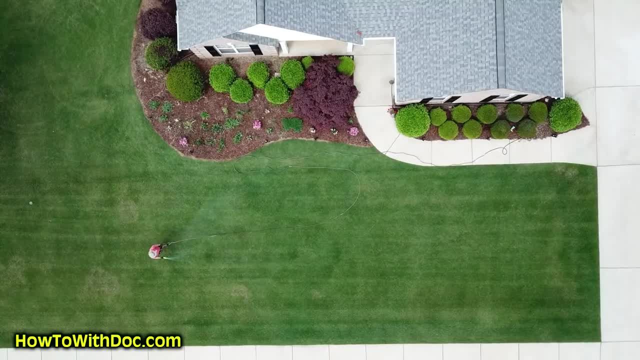 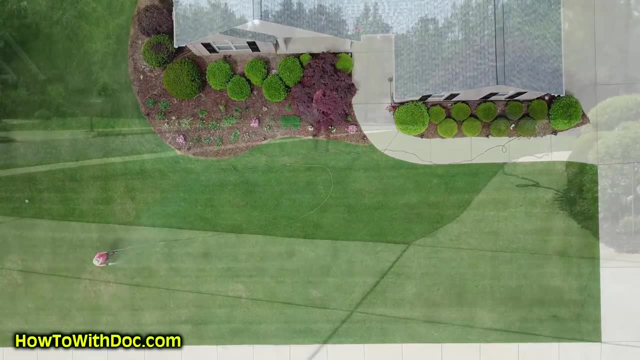 I'm just going to go ahead and spray it up, just to see if it's going to come off. I'm going to go ahead and spray it up, And that's it. Now I'm going to go ahead and spray it up, But if I fall, I will get up again.